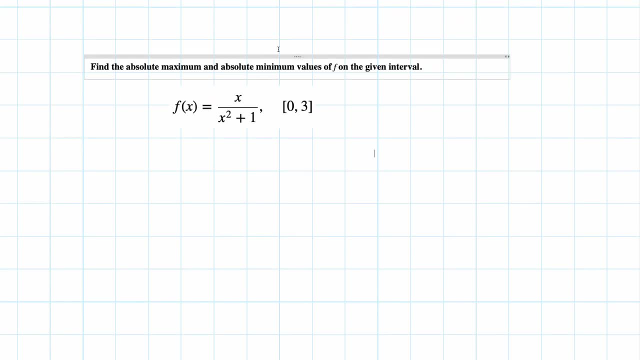 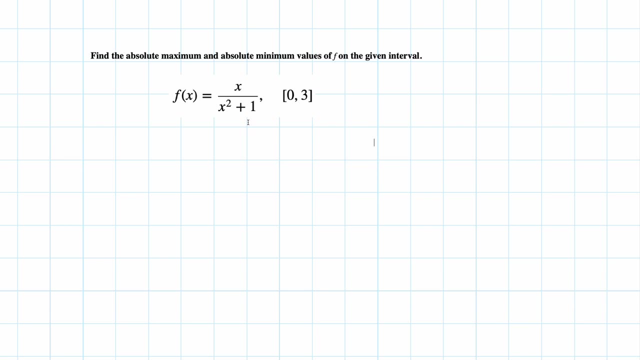 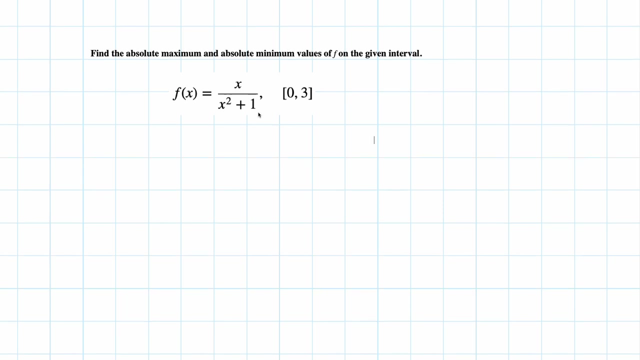 Find the absolute maximum and absolute minimum values of the function on the given interval, which is 0, 3.. So to find the absolute max and min, we need to find the critical numbers of this function. So critical numbers means we need to find the derivative and set it equals 0.. Okay, so let's do it. let's find the derivative. 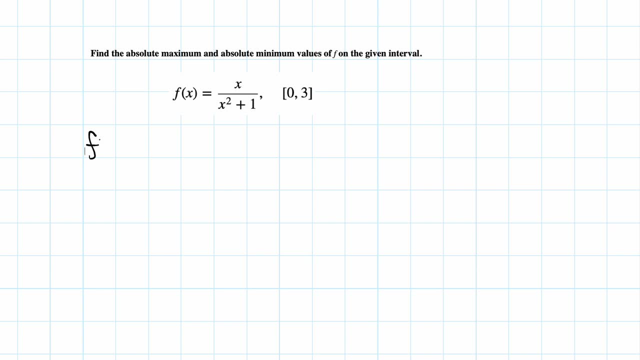 so this is a quotient, this is a fraction, so when we find its derivative we need to use the quotient rule. So when we have a function on the top, on the bottom, and when we find its derivative, that is f, prime g minus g, prime f over g square. So 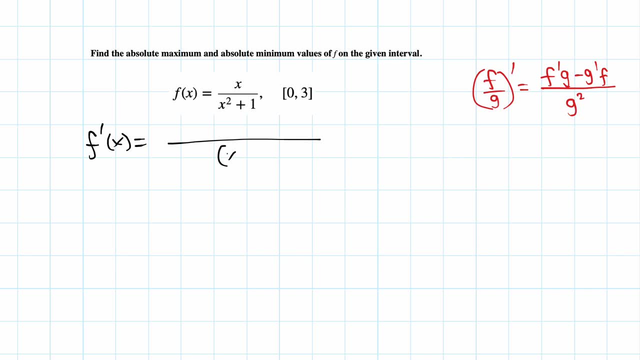 that is in this case on the bottom. bottom is square derivative of top times bottom, minus derivative of bottom, which is 2x times top. Okay, let's simplify 1 times x square, this x square plus 1 minus 2x square, all over x square plus 1 square, You can. 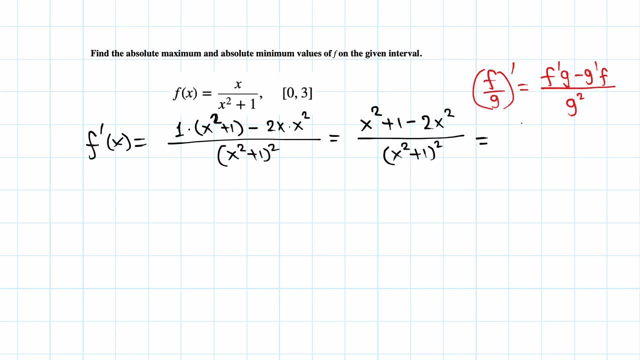 combine the x square and negative 2x square. Let me put: 1 minus x square. right x square minus 2 x square. 1 copy minus 2 copies negative, 1 copy left over x square plus 1 quantity squared. There are no cancellations and we know that the 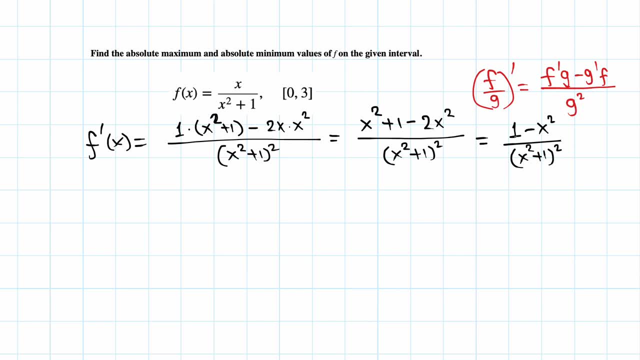 critical numbers are those x values where the derivative is 0 or where the derivative is undefined. In fact, on the bottom we got something square is a plus sign. so this is defined everywhere and we only, we are only interested in seeing inside 0, 3 anyways. so this is defined everywhere. So 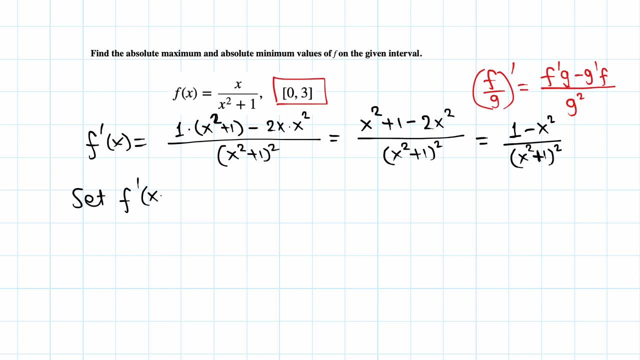 the critical numbers are just x values where the derivative is 0. now That means 1 minus x square over x square plus 1 quantity square equals 0.. Let's solve for x one fraction or 0. we can say 0 over 1. now let's do the cross. 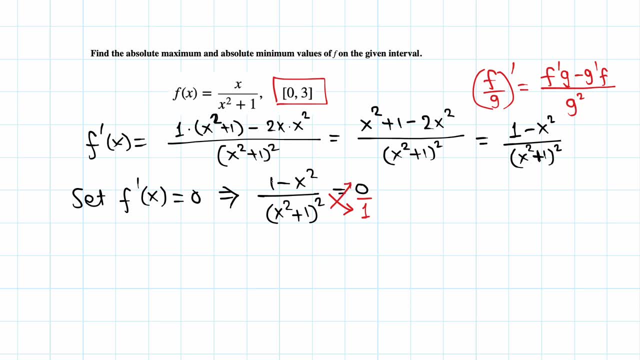 multiplication. That's how we get rid of the fractions 1 minus x square times 1. just 1 minus x square equals this thing: times 0 is just 0.. We have only two terms, so we can move one over or we can factor, so we have several ways to. 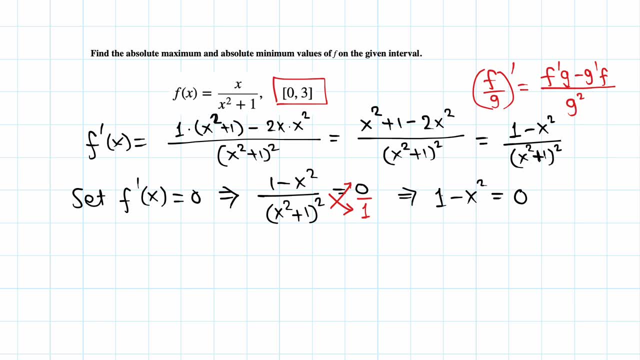 solve this. this equation: 1 is square minus x square. we can factor as well, if we like: 1 minus x. 1 plus x equals 0. from this, this is 0 when x equals 1, and 1 plus x is 0 when x equals negative 1.. 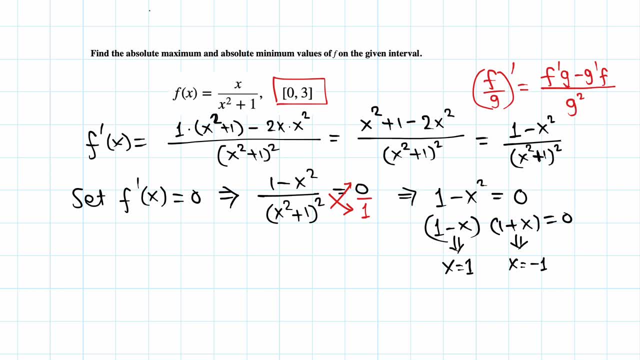 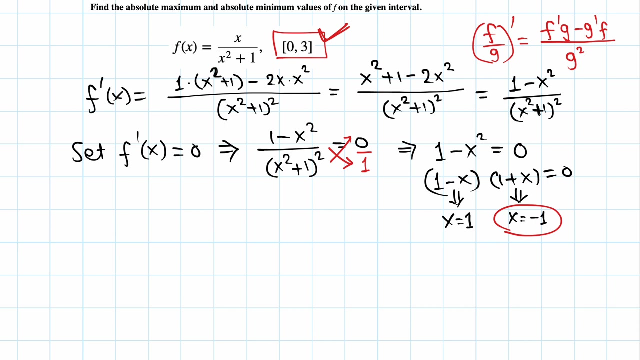 So these are two critical numbers, by the way, but our focus is here- 0, 3- and this negative one is not inside here, so we can disregard, we can discard this critical number for our purpose. okay, So now we evaluate the function to find the absolute value. 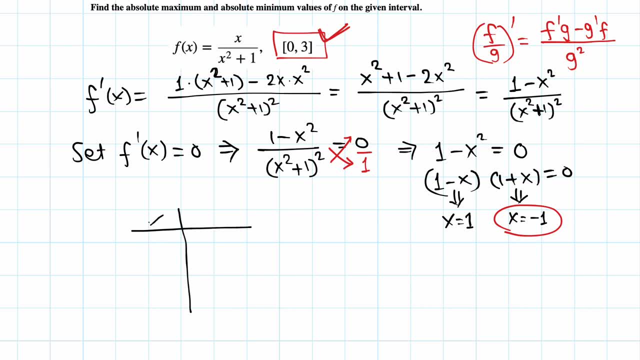 sorry, absolute maximum minimum. we just evaluate the function, which is x over 1 over x square plus 1,. okay, on the on this critical number one, and at the end points of the given interval, 0, 3.. Plug in 1 here, that means into the function. 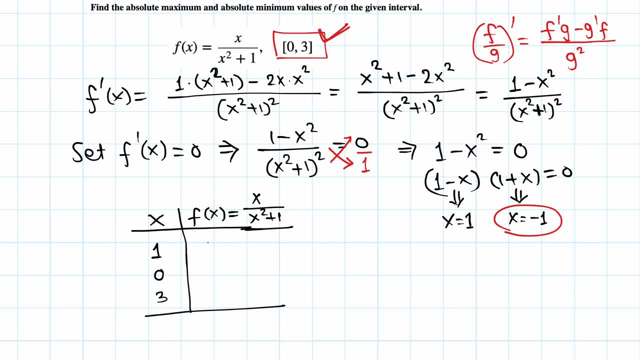 1 over 1, square 1 plus 1, 2, 1 over 2. 1 half Plug in: 0, 0 over 0, squared plus 1 over 1. just 0, 3, 3 over 3, squared 9 plus 1. 10, 3 over 10 and out of these three: